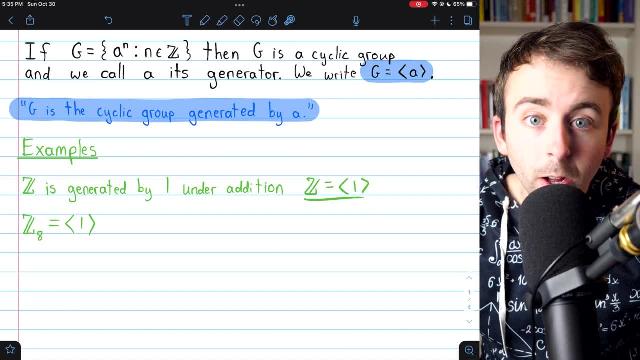 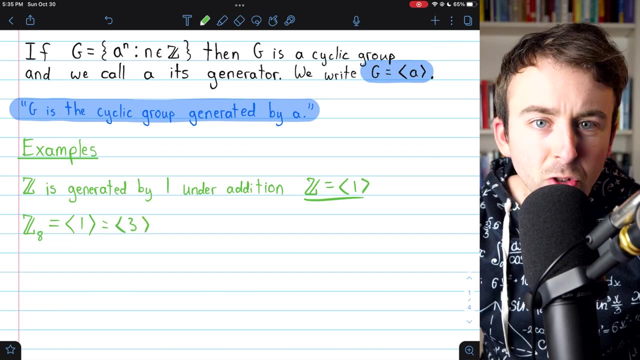 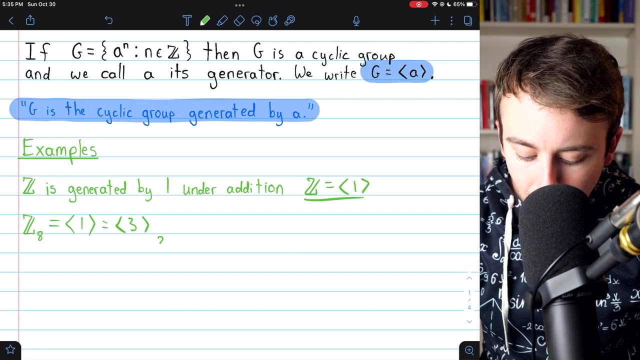 Another example is the integers mod 8. All 8 elements of this group are generated by 1. Interestingly, we could also generate this cyclic group with a different element, like 3, for example. Let's just check that by going through the multiples of 3 mod 8. The first multiple of 3 would be 3. Then we would have 6. Then we would have 9 mod 8, which is 1. 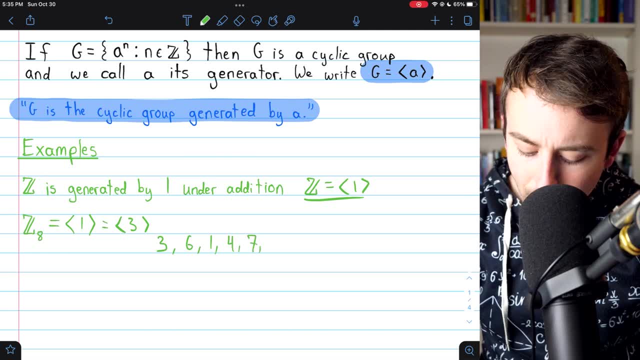 And then 4. And then 7. And then 10 mod 8, which is 2. And then 5. And then 8. 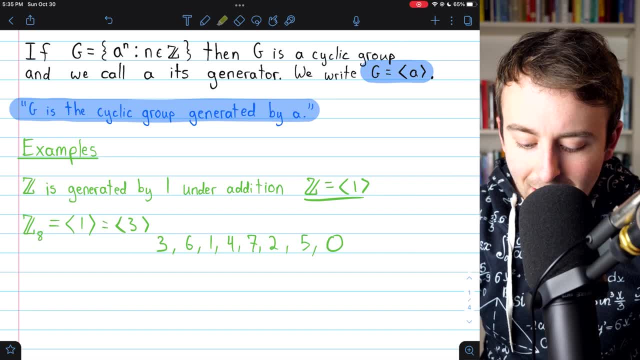 Which, of course, mod 8 is 0. So we see how the multiples of 3 generate the entire group of the integers mod 8. 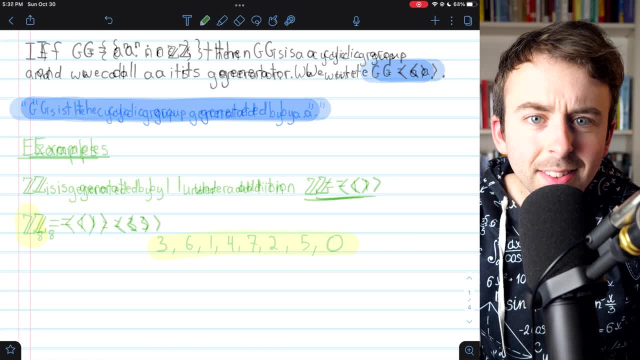 Indeed, they are generated by 1 and 3. See if you can find a third generator for the integers mod 8. 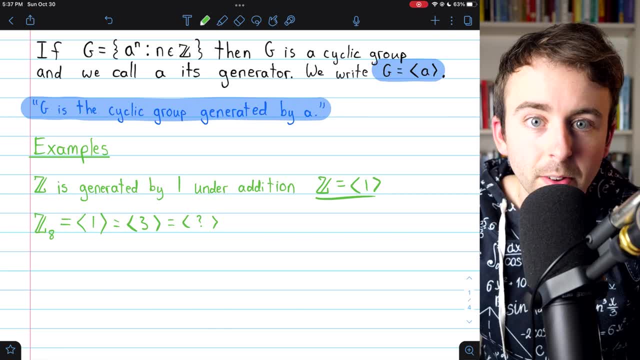 Next, we're going to move on to discussing an isomorphism concerning cyclic groups. 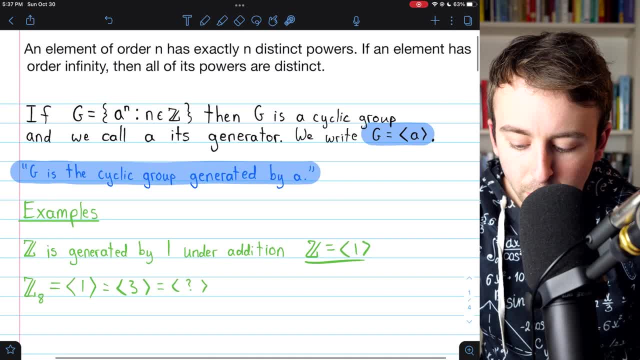 For that discussion, it will be important that you're familiar with this result. 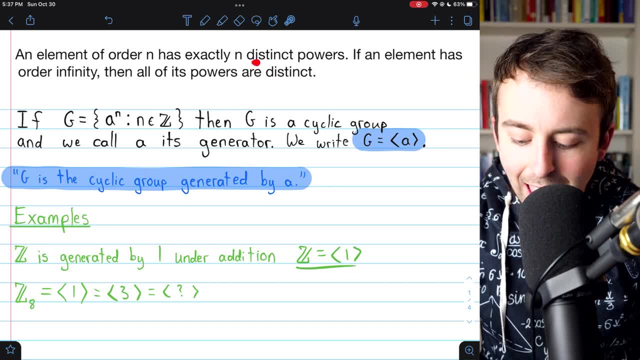 That an element of order... ...has exactly n distinct powers. 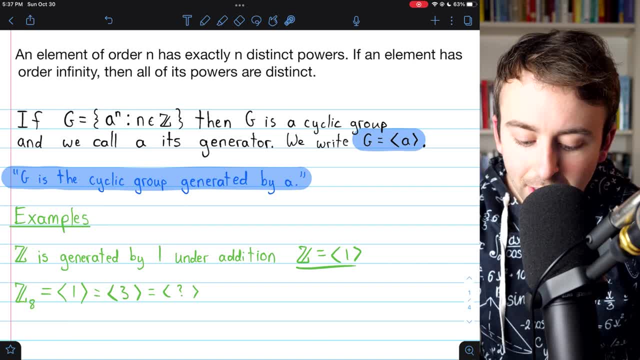 And if an element has order infinity, then all of its powers are distinct. I'll leave links in the description to my lessons proving these results. 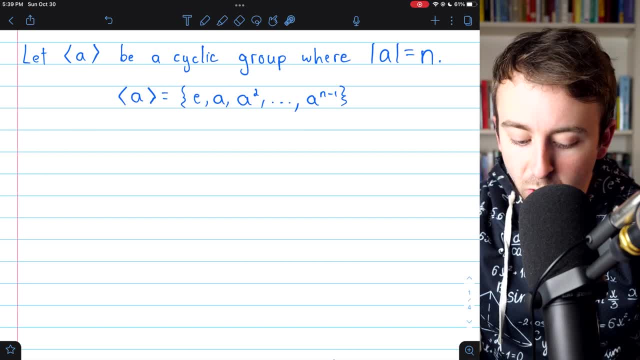 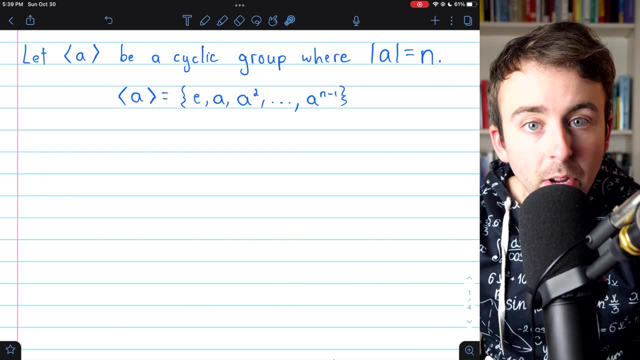 Okay, let A be a cyclic group generated, of course, by A, where A has order n. That means this cyclic group generated by A will have the n distinct powers of A... ...from the identity element E, or A to the 0, all the way through A to the n-1. 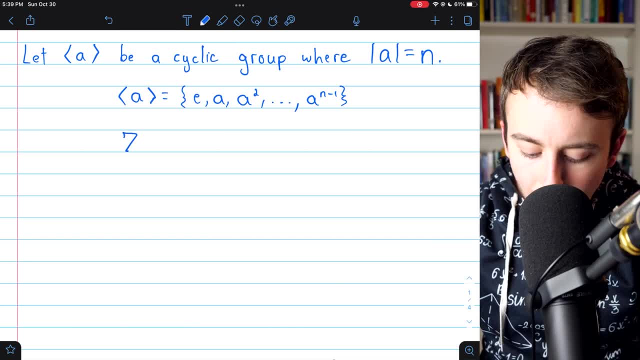 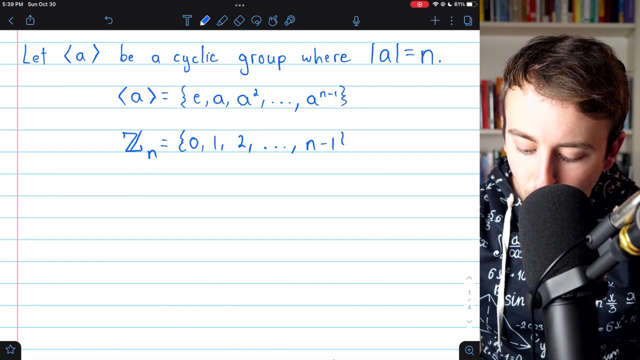 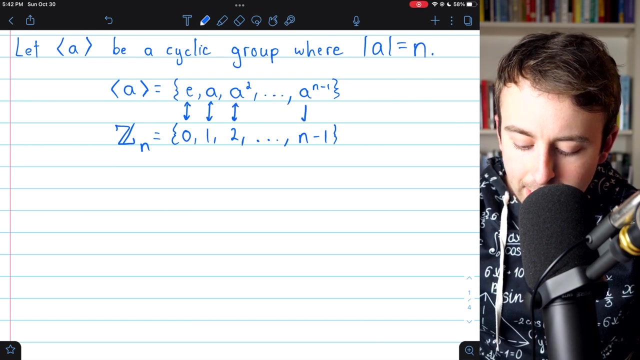 Then, we could consider a correspondence with this cyclic group and the integers mod n. The integers mod n, of course, contain 0, 1, 2, and so on, all the way through n-1. It is plain to see that there's a bijection, a 1-1. There's a 1-1 correspondence between these two groups. 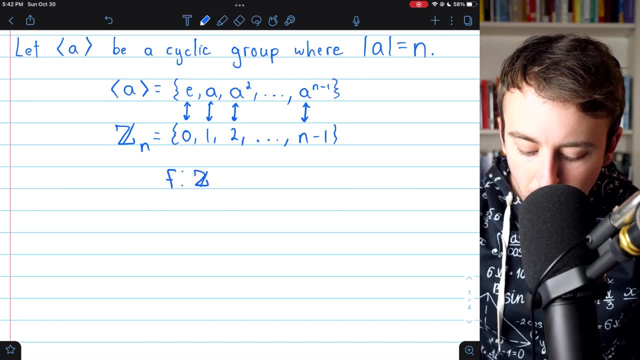 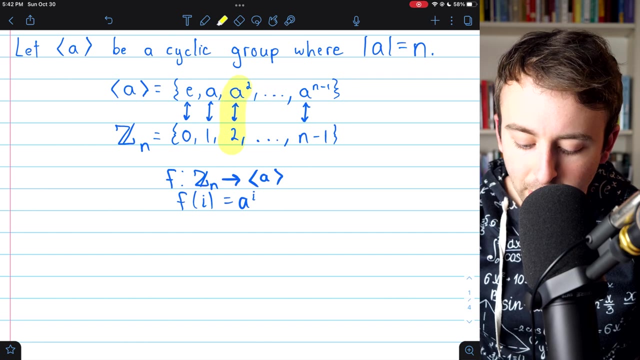 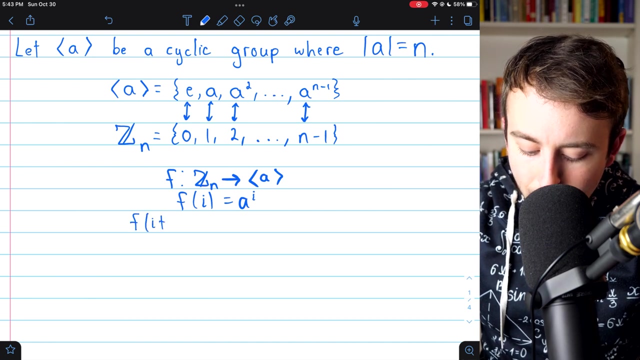 We could say that this function maps the integers mod n onto the cyclic group generated by A. And the function is defined like this. f of i is simply equal to A to the i. f of 2 brings us to A to the 2, for example. This function has an interesting property, which is that f of i plus j... 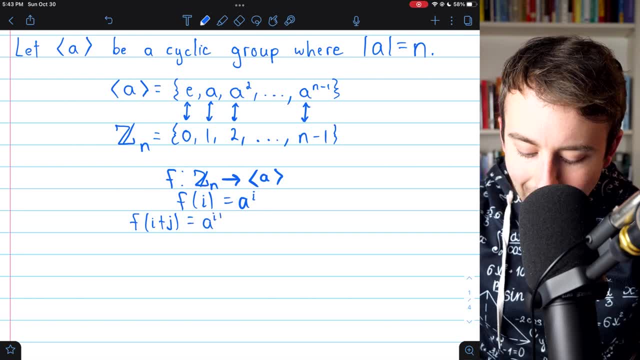 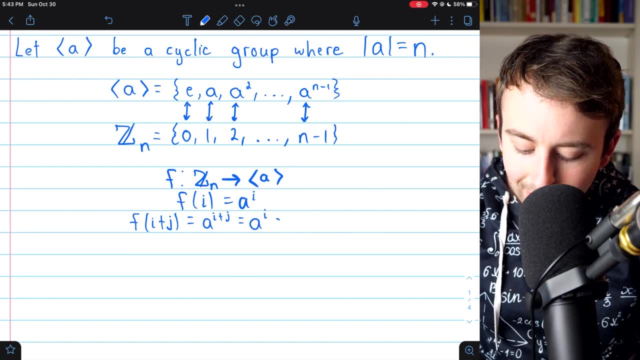 ...by the function's definition, is equal to A to the i plus j. But then, by our exponent laws, A to the i plus j is the same as A to the i times A to the j. But then again, by definition of our function, that's equal to f of i times f of j. So, in fact, by definition, this bijection between the groups is an isomorphism. Let me take a look at this. 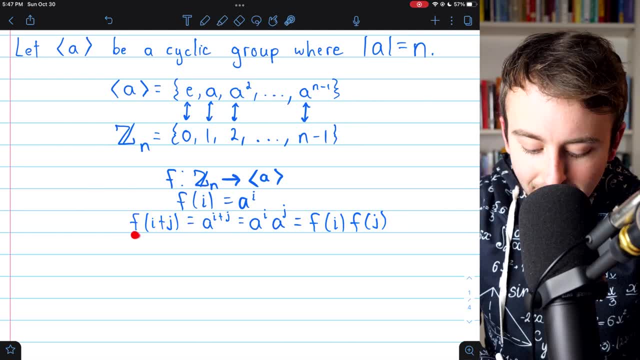 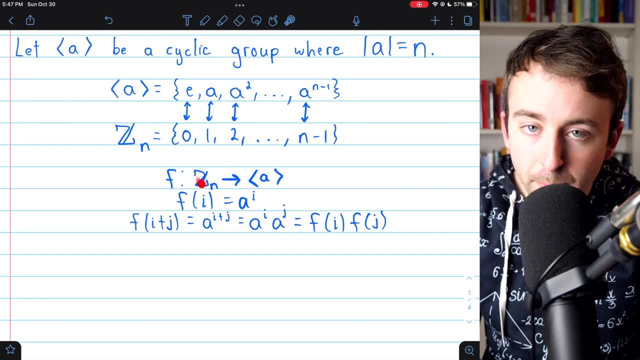 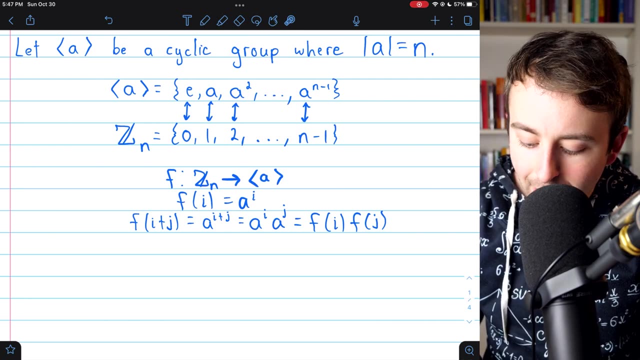 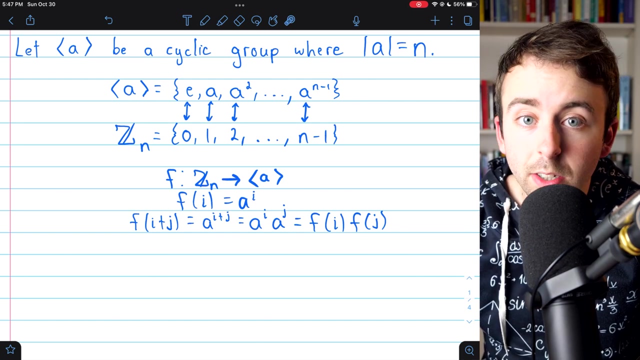 Let me take a moment now to discuss notation. See, inside the function, we wrote i plus j, because i and j came from the integers mod n, which we are treating with the operation of addition. However, we write f of i times f of j, because for the cyclic group generated by A, we've chosen to use the multiplication notation. 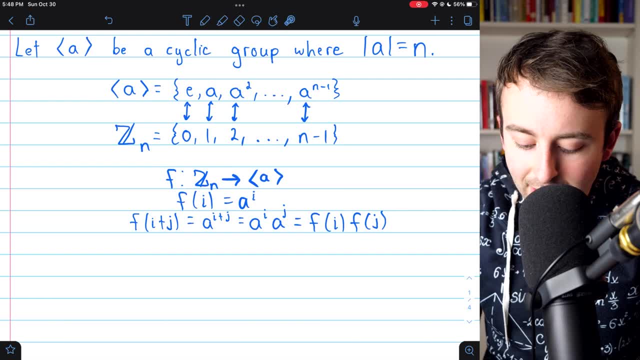 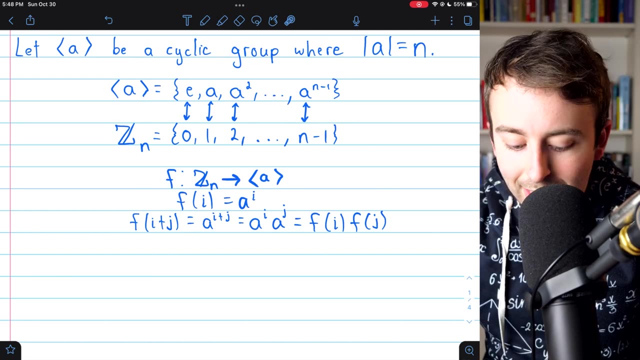 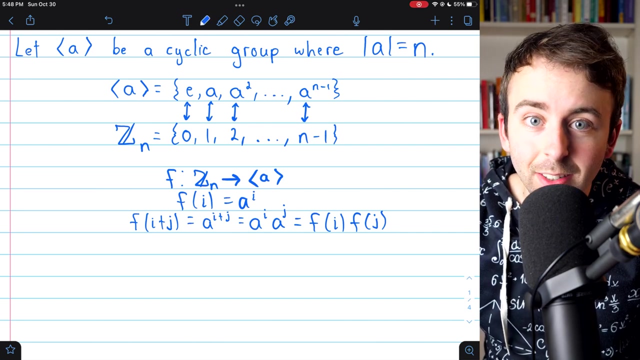 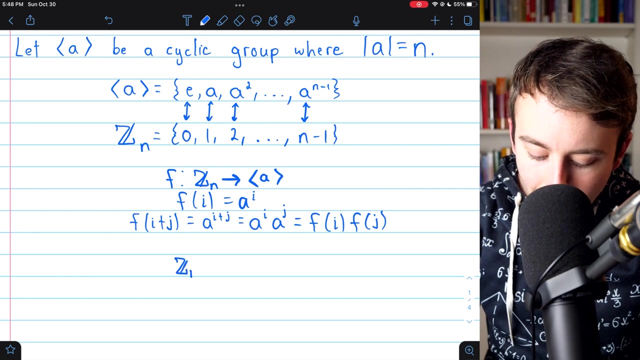 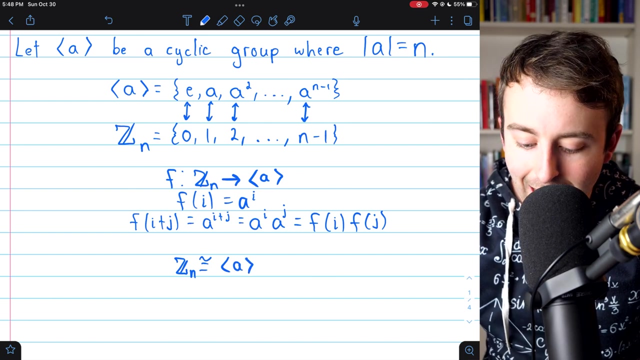 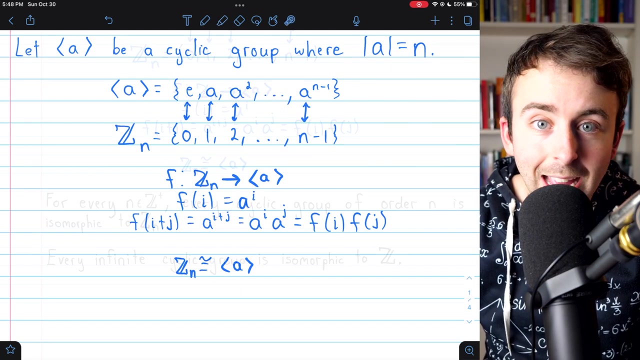 Regardless, we see that combining the elements... ...in the integers mod n, so doing i plus j, and then sending it through the function, gives us the same result as sending i and j through the function first, and then combining them under the operation that is in the cyclic group generated by A. So, by definition, this is an isomorphism. It does what we sometimes call preserves the group operation. So, we could write that the integers mod n... ...are indeed isomorphic to this cyclic group of order n generated by A. And the only thing we assumed about this cyclic group was that it's generated by an element of order n. So, here are our big takeaways. 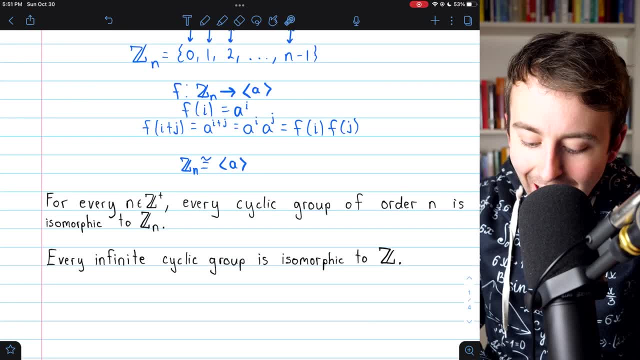 For every positive integer n, every cyclic group of order n is isomorphic to the integers mod n. Pretty cool. 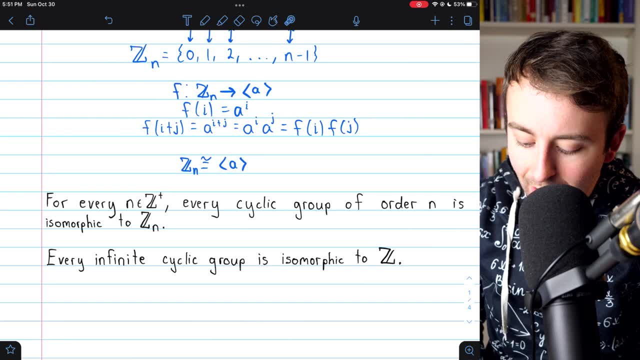 Similarly, every infinite cyclic group... ...is isomorphic to the integers. 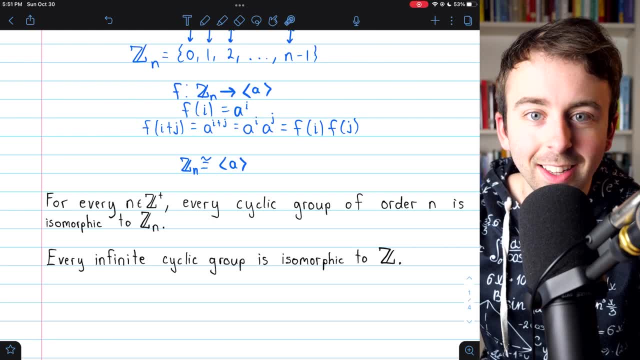 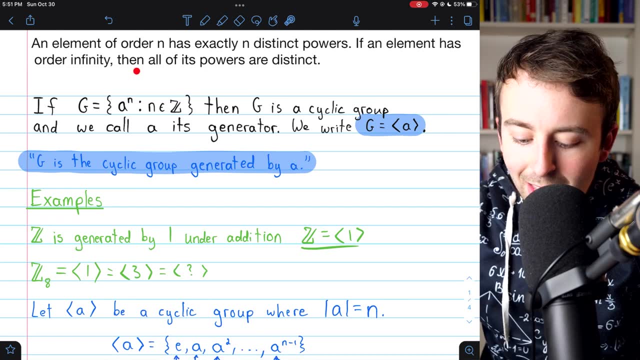 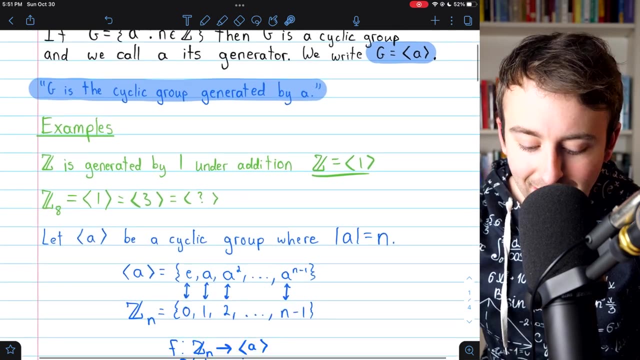 This is a very similar result, so I'm not going to go through the details here. You would just need this result I mentioned earlier, that if an element has order infinity, then all of its powers are distinct. That way, you would be able to draw a bijection from the infinite cyclic group it generates to the set of integers. 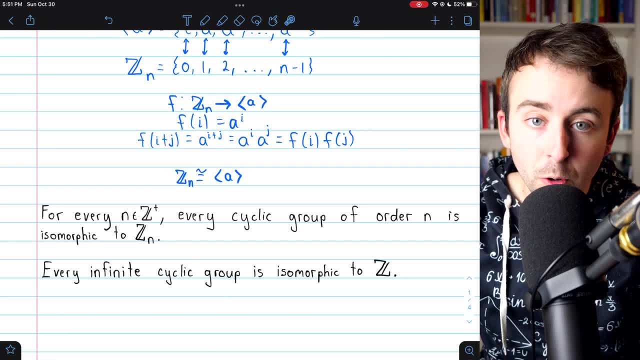 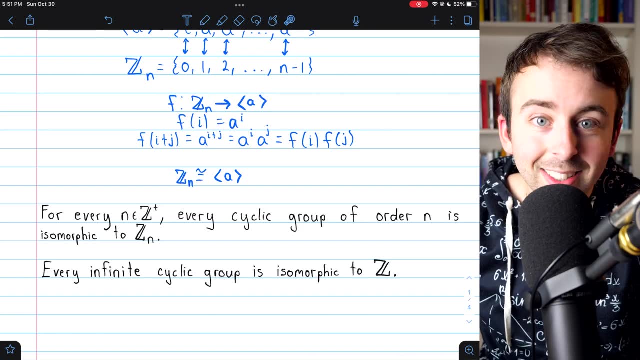 This, of course, also means that every infinite cyclic group, any two infinite cyclic groups, are, in fact, isomorphic to each other, because they're all isomorphic to the set of integers. One more thing before we go. 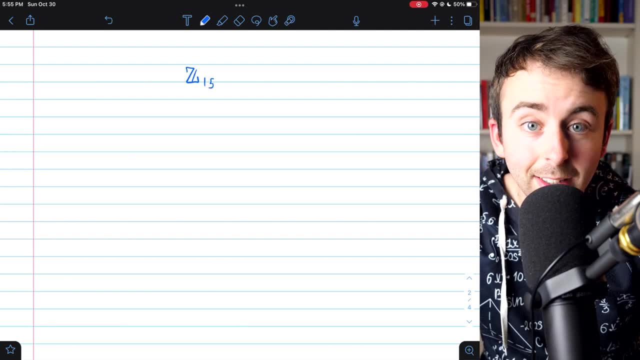 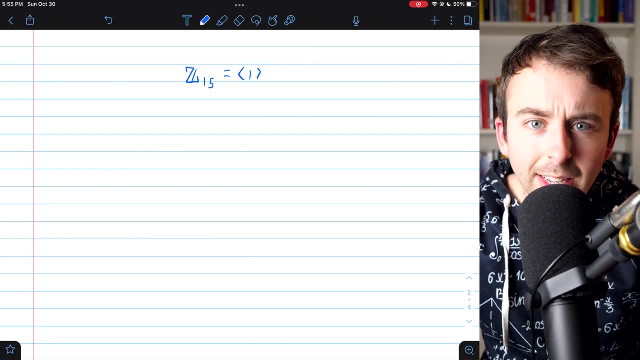 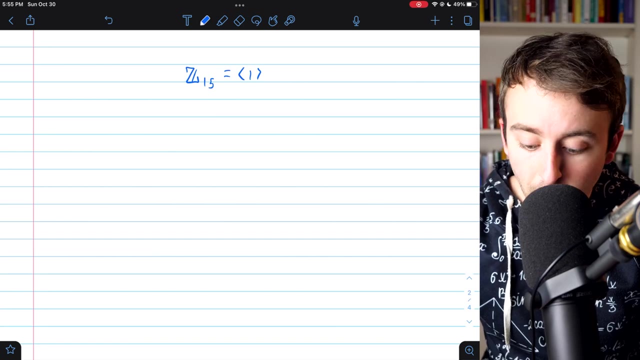 Certainly, the integers mod 15 is a cyclic group. For example, it's entirely generated by 1. But it also contains some subgroups that are cyclic. For example, consider the powers of 3. The 0th power, or in this case, we're talking about addition. So, let's say 0. 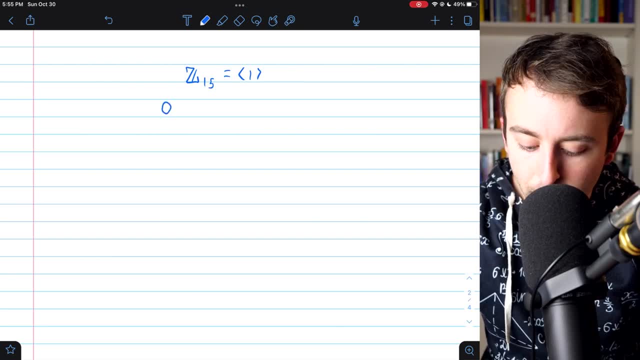 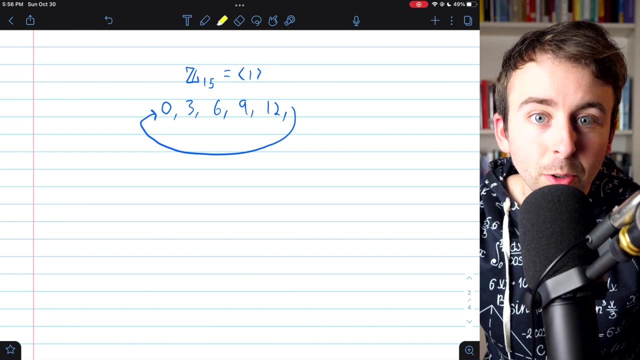 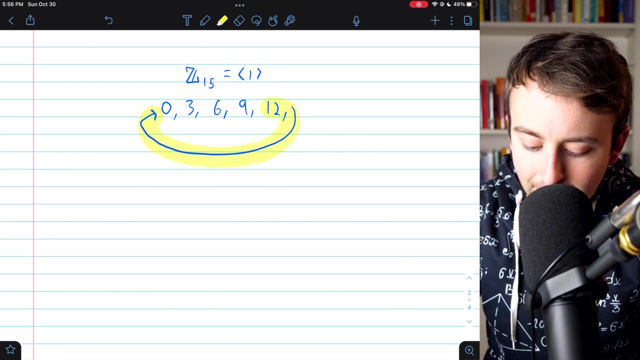 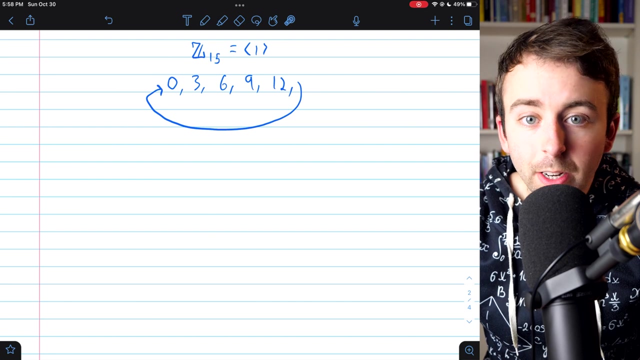 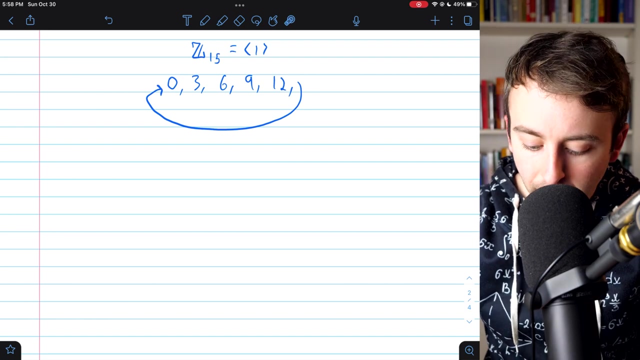 Let's say multiple. The 0th multiple of 3 would be 0. Then 3, then 6, then 9, then 12, and then 15, which is 0. So we'd actually just come right back around. If it wasn't already clear, that's why these are called cyclic groups. Because, at least in the case of finite order, a generator will eventually complete an entire cycle, and then just keep looping through the group repeatedly. A couple things you might notice here is that if we combine any of these multiples of 3, we get another multiple of 3. 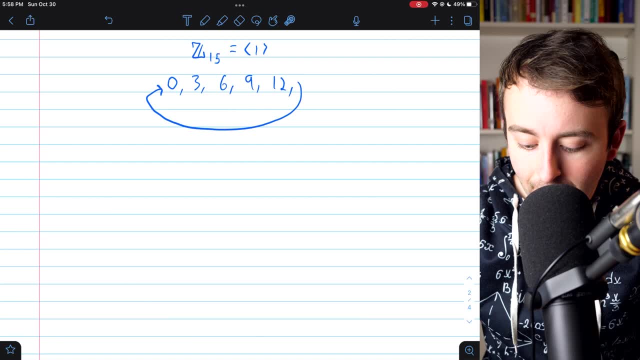 3 plus 6, for example, brings us to 9. 9 plus 12 brings us to 21. 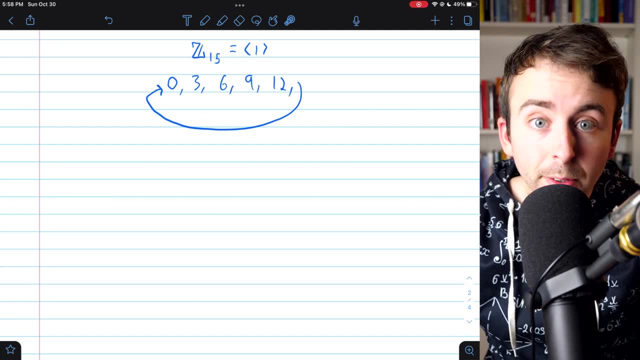 Mod 15 is 6. If we combine multiples of 3, we get another multiple of 3. 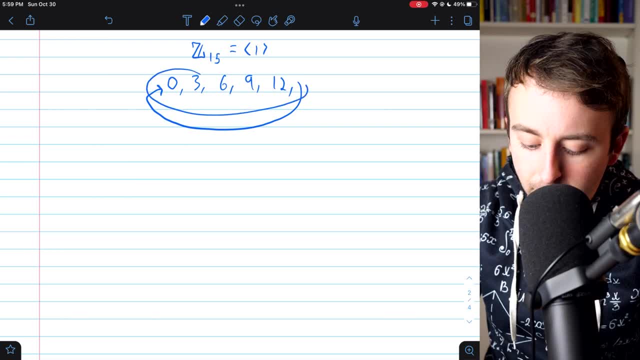 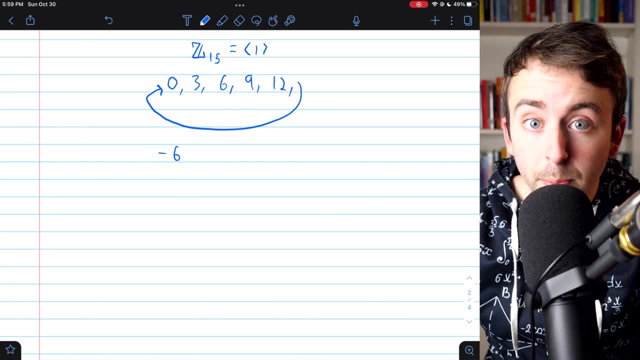 The second thing you might notice is that if we take the inverse of any of these multiples of 3, like negative 16, for example, this is also a multiple of 3. 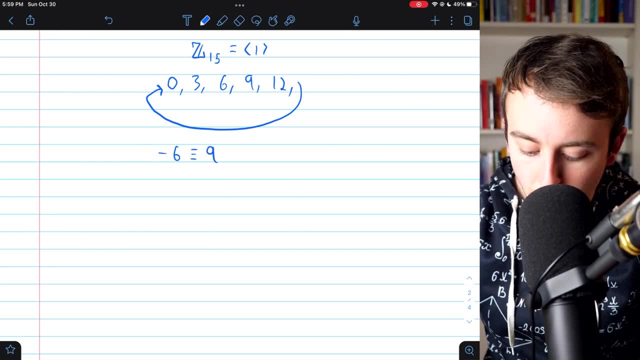 Negative 6 mod 15 is congruent to 9, the third multiple of 3.